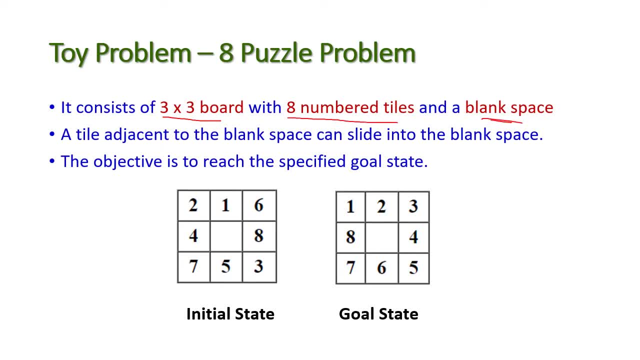 with a blank space. So this is the 8th puzzle problem. See, this is the board of 8th puzzle problem. This board is having 9 different blocks, that is, 3x3 board 1,, 2,, 3,, 4,, 5,, 6,, 7,, 8,, 9.. So 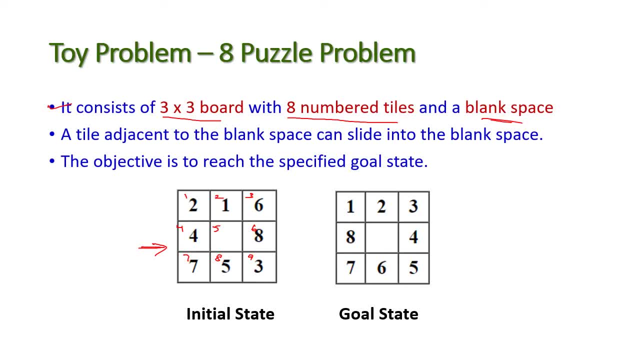 totally. 9 blocks are there. So in these 9 blocks, 8 blocks will be occupied by numbered boards, numbered tiles, Okay, and only one blank space is there, and this is the blank. Okay, and the tile adjacent to the blank space can slide into the blank space. Okay, the tile adjacent to the blank space. 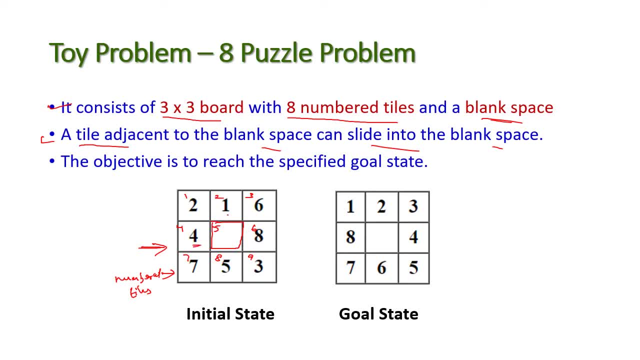 which are the adjacent tiles here. So these tiles may be come towards the blank space and the objective is to reach the specified goal state. Okay, in the problem itself they will give the initial state and goal state. So from the initial state we need to reach the goal state while moving these tiles towards. 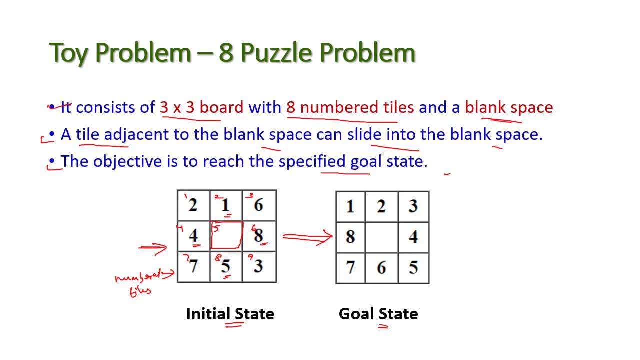 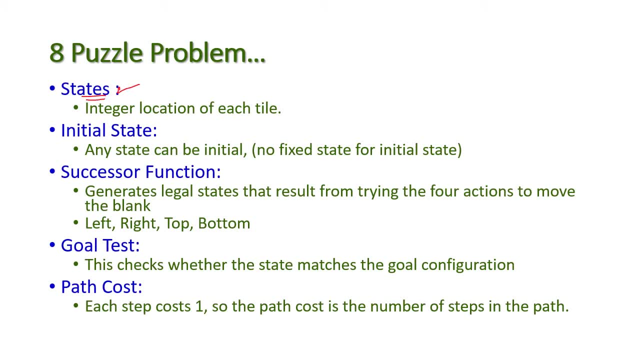 the blank space. Let us see how to solve these problems. Let us see how to solve these problems. Let us see how to solve these problems. Here we should find the states. What is states here? The integer location of each tile? Okay, 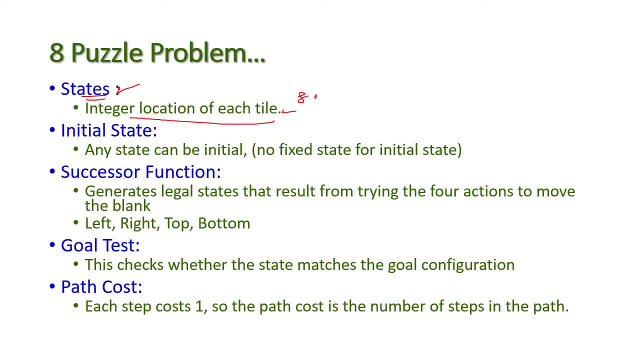 we are having 8 numbered tile, 8 numbered tile and these numbered tile will be located in which block Block position in the board. So this is called as state and next one is initial state. This may be any state and that will be given in the problem itself. There is no fixed initial state, Right and next. 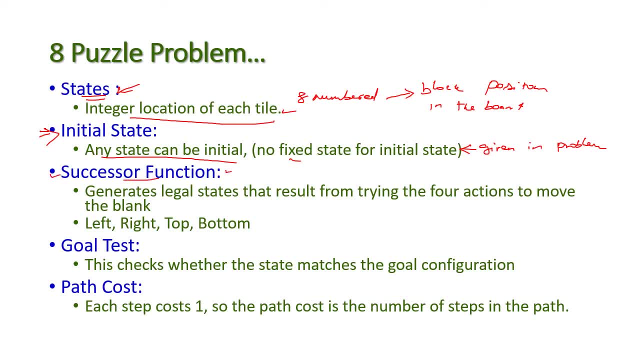 one is successor function. In the successor function it generates legal state that results from trying the four additional functions. This is called as state. Under the first function, this is called as state. This is called as state. Under the second function, this is called as state. 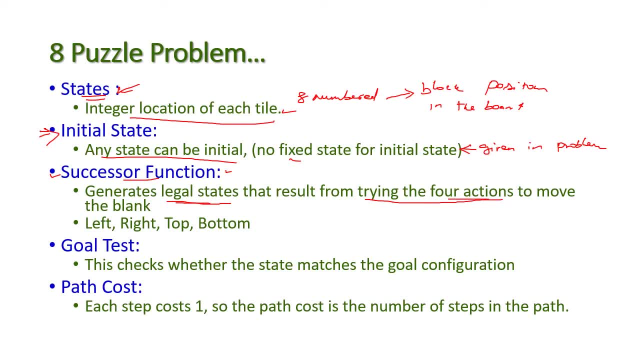 actions, four actions. what are the four actions we are having? move left, move right, move top, move bottom. that is, the blank will be moved from any of the direction: left to right, top or bottom. so by using this, the successor function will get generated. and next one is goal test, and this is: 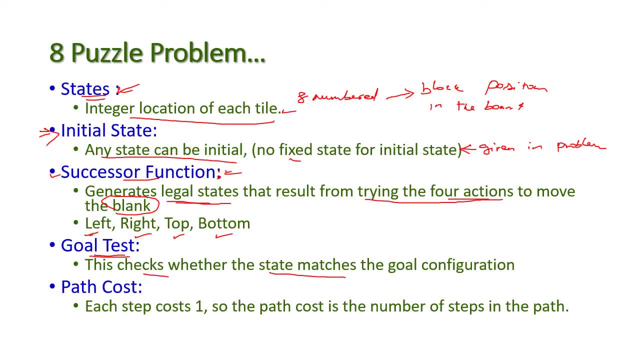 used to check whether the state matches the goal configuration or not. the goal will be given in the problem, given in problem problem itself. right, so we know what is goal for this ital problem and at the every state we need to test whether the goal is matched to this state or not. that is the 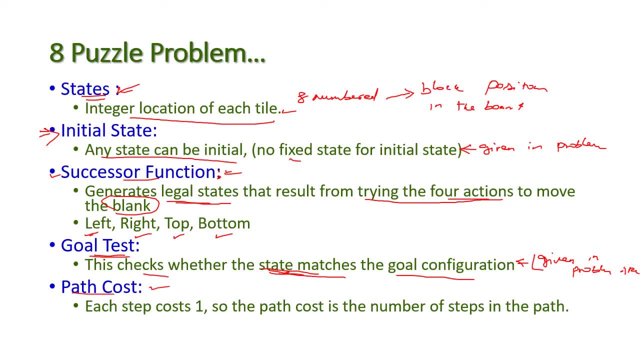 current state or not. and next one is path cast. each step cast is one, okay, so they didn't give any cost of the movement, so default is one, and so the path cast is number of steps in the path between start state to goal state. okay, how many movement are there from start state to goal state will be computed for this cast, step cast. 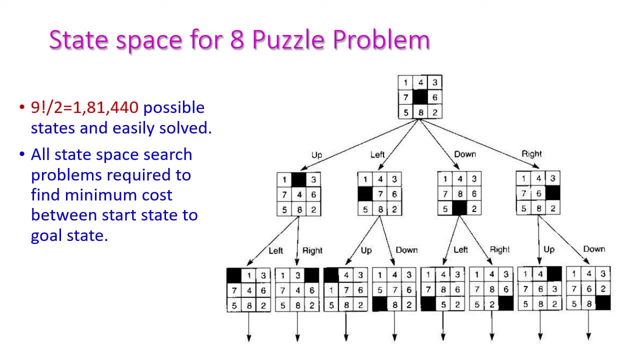 and the state space for eight puzzle problem. here we are having nine blocks, so total number of states will be nine, factorial by two, and this number is one lakh eighty one thousand four hundred and forty possible states, and those are easily solved. okay, anyone can easily solve this eight puzzle problem. 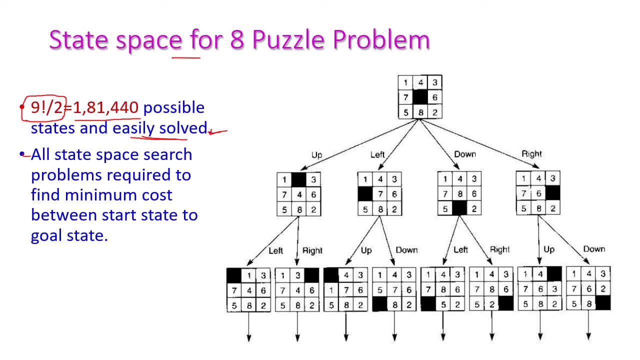 here requires to find minimum cost between the start state to goal state. okay, so this is the state space search tree search tree for this 8 puzzle problem. so this is the initial state. this is the initial state. so from the initial state we are going to generate the 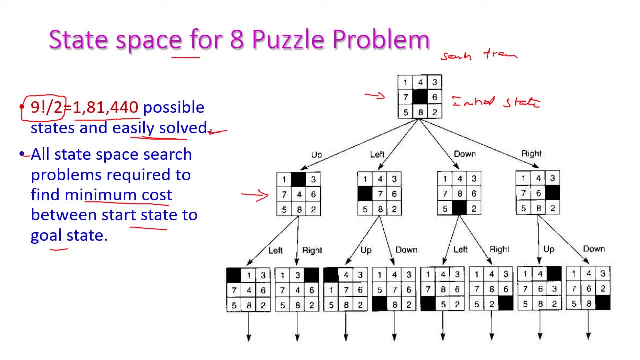 adjacent states. for example, this is v naught and this is v1 right in the v1. what are the possible states there? we can move this 4 downward direction so that the blank will move go up. otherwise we can move 7 in the left direction- sorry, right direction- so that the blank will move. 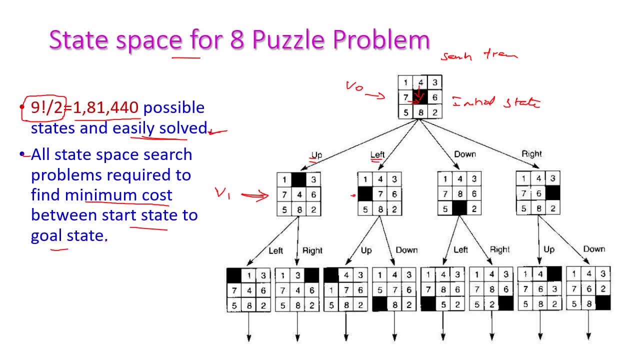 left. otherwise we can move this 8 upward direction so that the blank will goes down. otherwise the 6 will be moved to the left direction so that the blank will moves to the right. so likewise we can generate. so this is v2. likewise we can generate so many. 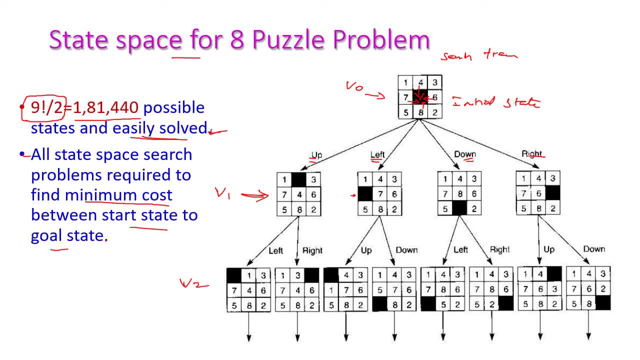 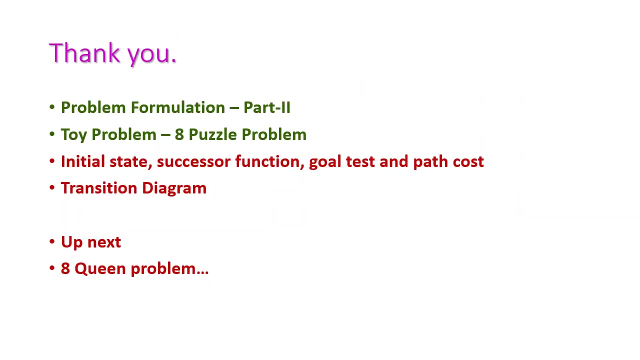 state space search tree. we can generate this tree, and this will go on until we reach the goal state. okay, and finally we need to compute the path cast. path cast- okay, how much cost it will take from start state to goal state? okay, and that's all about 8 puzzle problem in this class we have seen. 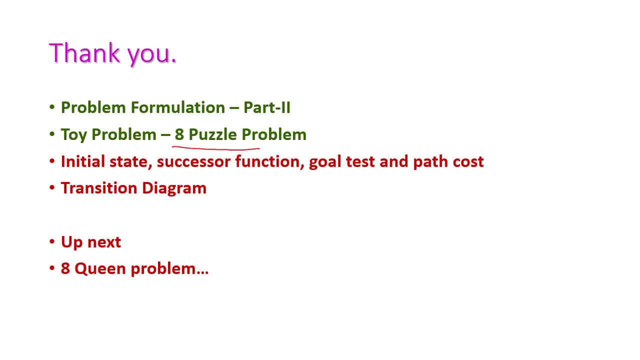 uh, the 8 puzzle problems: initial state and final state. okay, and finally, we need to compute the path set, successor function, goal test and path cast, as well, as we drawn this transition diagram, which is otherwise called as state space search tree, to find the goal. okay, to find the goal, and this is. 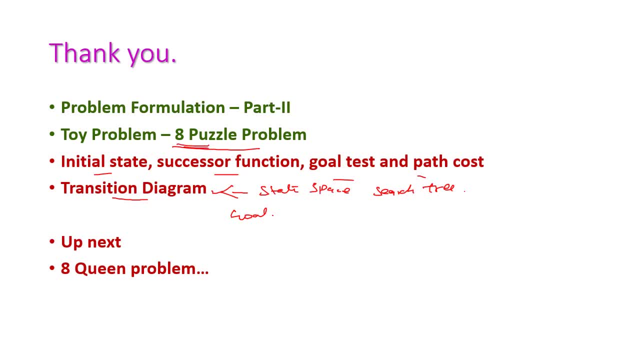 very simple problem and in the next class we will see the 8 queen problem and if you have any doubt you just text me. otherwise you can give your comment in the comment box. thank you,